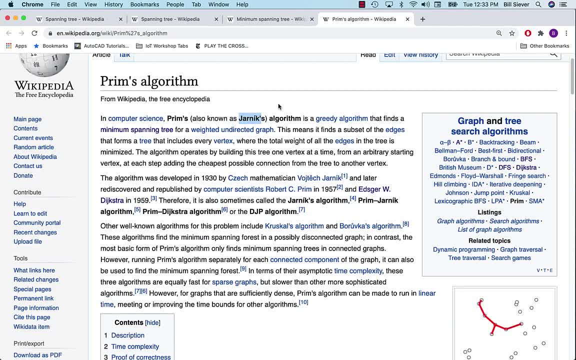 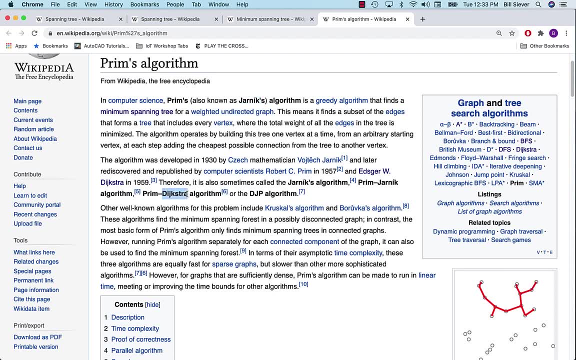 So, first off, Prim's algorithm was actually invented by Jernick before Prim, or at least discovered. So multiple people get credit for this, including Dijkstra. So this is a well-known algorithm. It's been discovered and rediscovered multiple times. 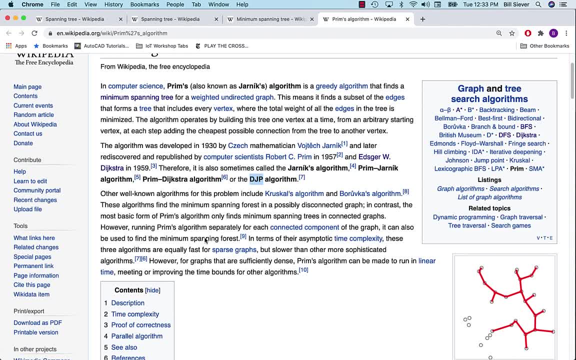 You could even call it the DJP algorithm. Okay so, there are also other well-known algorithms, including Kruskal's algorithm, which we will also look at. Okay so, let's take a quick look at basic structure of Prim's algorithm. Okay so, Prim's algorithm is similar to an. 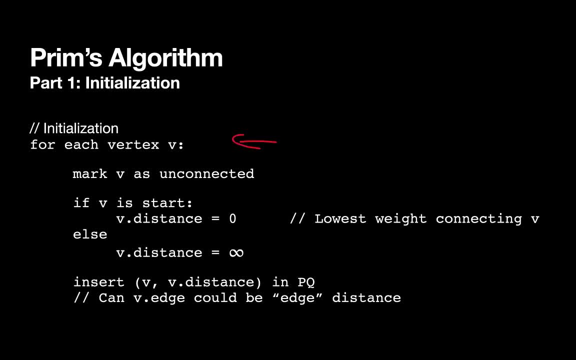 algorithm that we've seen in the past. It processes vertices, so it's got a loop that will loop through and initialize each vertex. First off, it's going to somehow indicate that it's unconnected, And then we've got some sort of start vertex And again- remember, we're creating a spanning tree- It's eventually- 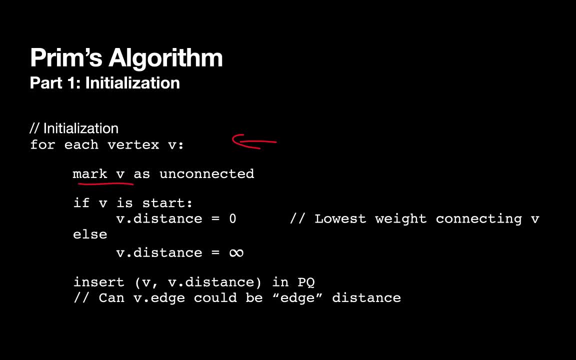 going to hit every vertex, so it really doesn't matter where we start. So if we're at our start, we'll indicate that its distance is zero. Otherwise we'll update its distance to be infinity. So we're going to assume that we can't reach everything and we'll slowly 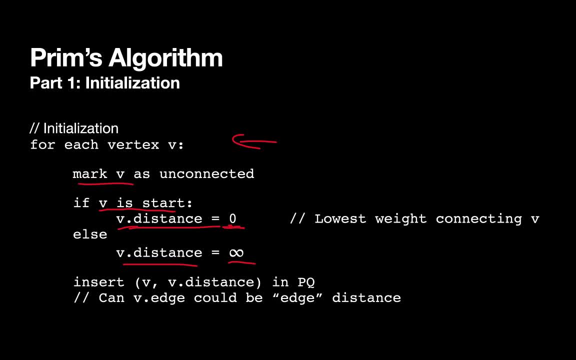 kind of expand out from our start, figuring out what we can reach. Okay, so we will insert all of our vertices into a priority queue At this point. we could also keep track of edges by somehow having an edge associated with a vertex. So basically, 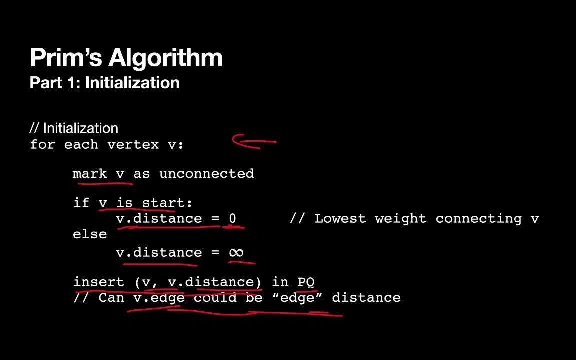 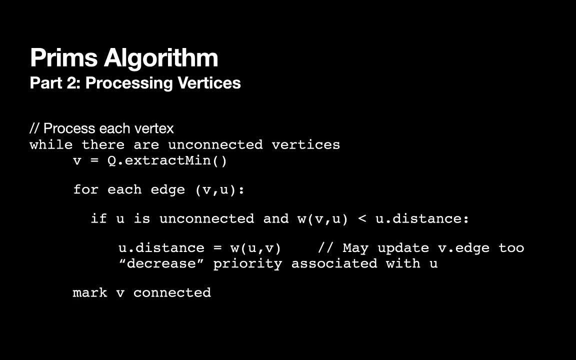 the edge would be the edge that is kind of the incoming edge in our spanning tree. Okay, so this is the initialization step. Next we go through and we process vertices. So we're going to continue going while there are still vertices that are not connected. 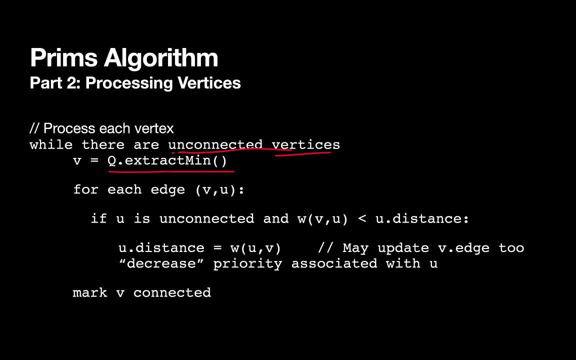 We'll continually extract vertices from our priority queue, so we'll get them kind of in order of the lowest cost, And then we'll go through each of their outgoing edge—the outgoing edges of our vertex- And we'll see if the outgoing edge is connected to something. 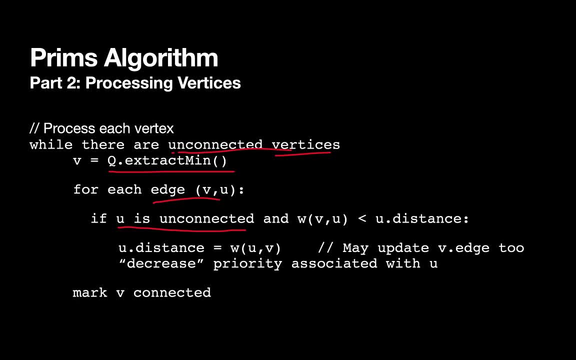 that's not yet connected to our spanning tree. And if so, we'll use that outgoing weight, that outgoing edges weight, to see if it's a good path, if it's better than the best known path, And if so, we'll get that spanning tree connected with something that it as far or 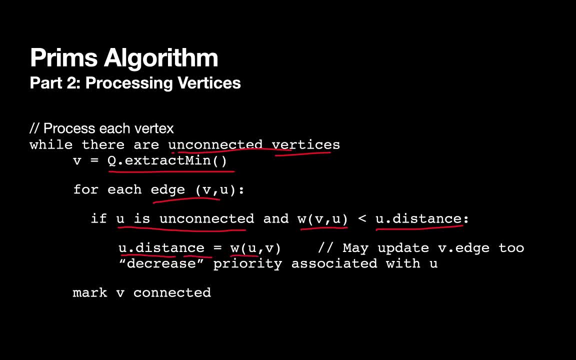 we'll update the overall distance that we can achieve to get to this new node on the opposite side of our V node and update the corresponding priority. by the way, this would be kind of the step where you keep track of the edge that's being used as well. so if you're truly building a spanning tree, you're mainly focusing. 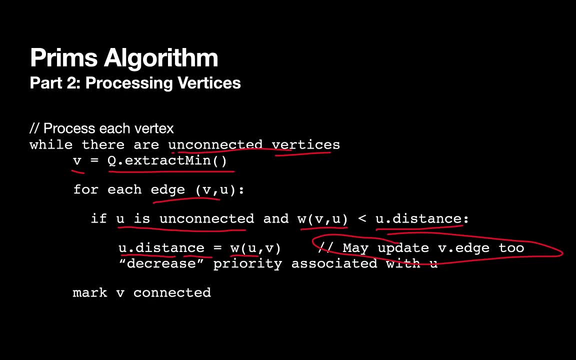 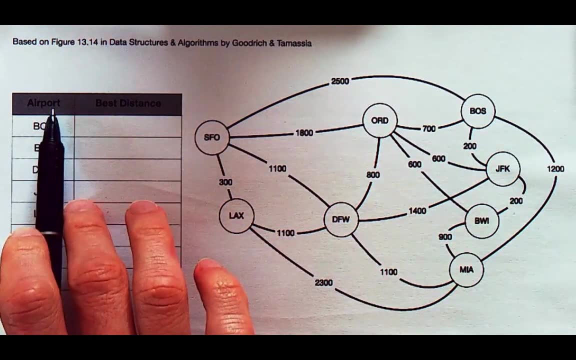 on constructing a set of edges, and this is one of the places where you're changing which edge might be selected for your final set of edges. okay, so let's go ahead and work through the example that we've seen before. okay, so here's our familiar problem again, our power line sort of graph I'm going to 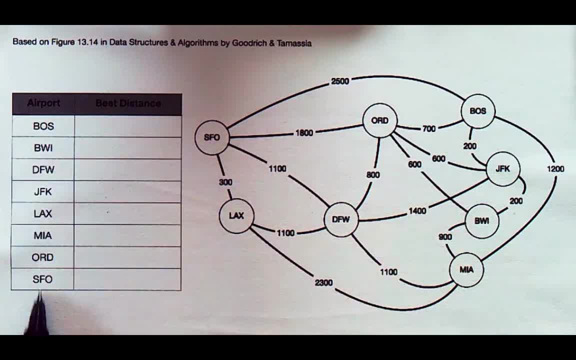 use this table here to represent my priority queue. so it's a table of the vertices and I'm keeping track of the corresponding distance which will represent the priority. also, I'm just going to kind of mentally keep track of which edges get used. in reality, as we'd be updating the distances here, we would 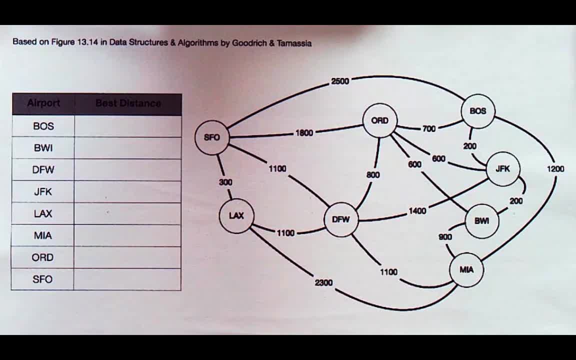 also somehow keep track of the edge that's capable of achieving that distance. okay, so step one: initialization, initialization, initialization. Again, I'm going to start out at San Francisco, so I'll initialize it to be a distance of zero. I'm going to check off the cities once I've actually connected them to my graph. 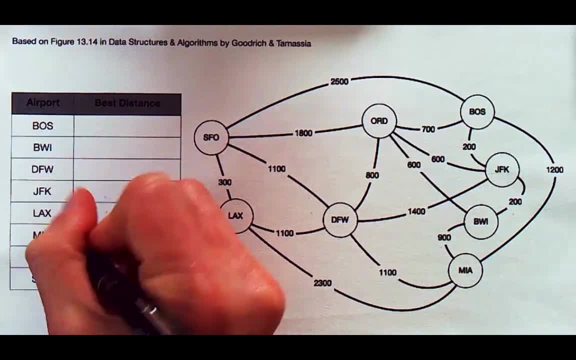 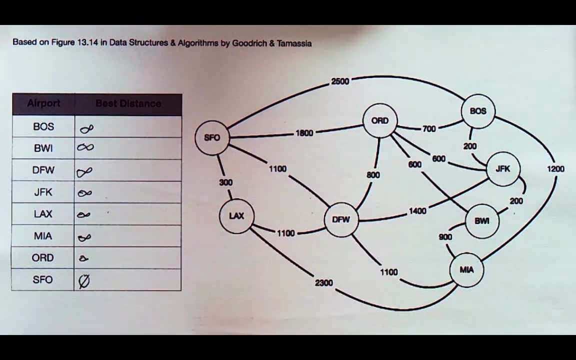 I'm going to go ahead and initialize everything else to be an infinite distance away from San Francisco as far as I know. And now we get to the body of a loop of Prim's algorithm that removes a vertex from the priority queue with the highest priority. 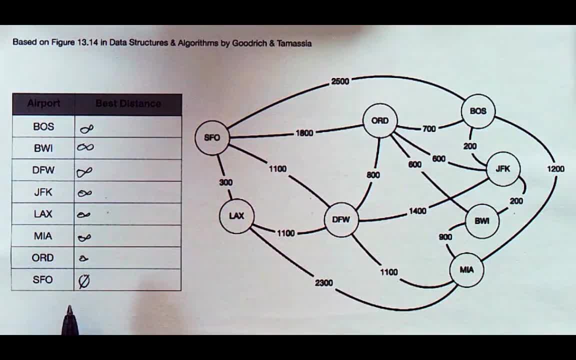 which will be San Francisco, And then it'll look at all of the outgoing edges and the opposite vertex and updating our estimates of distance to that vertex, at least if the vertex is still unconnected. So from San Francisco we'll look at all of our outgoing vertices. We've got, I'm sorry, outgoing edges. 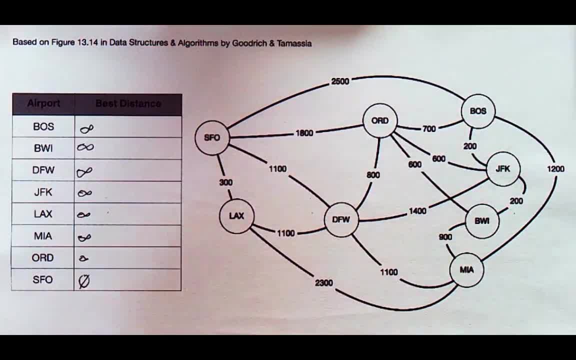 We've got an edge going to Boston. We can get to Boston with a total of twenty five hundred, So we'll go ahead and update our distance there. We've got an outgoing edge to O'Hare, So we'll go ahead and update that as well. Eighteen hundred: 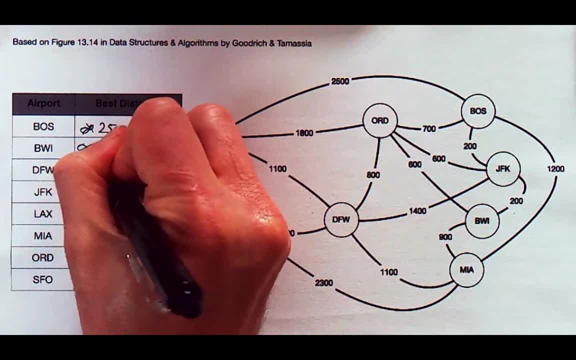 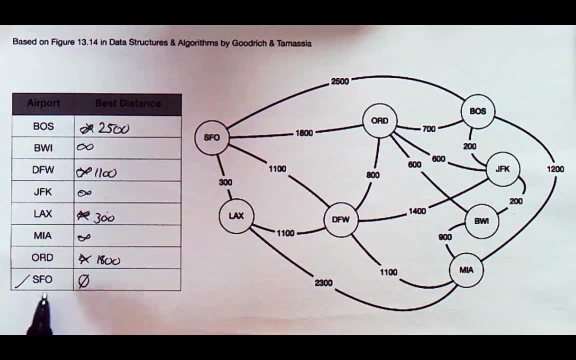 We've got an outgoing edge to Dallas of eleven hundred. We've got an outgoing edge to LA of three hundred. So we've now processed San Francisco. so we'll mark it as being connected. OK, now we'll repeat the process. So we'll remove our highest priority item, which is LA. 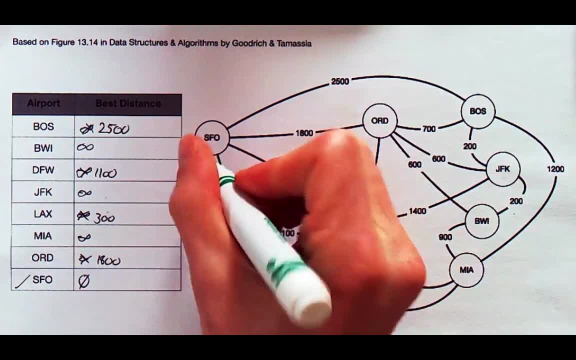 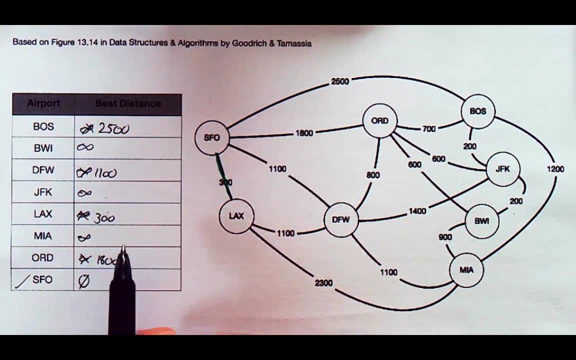 I'm also again going to kind of mentally keep track of which edges are being used. In reality, when I selected the three hundred, I would have stored away which edge was capable of achieving that. OK, so we'll process LA. We'll look at all of its outgoing edges. 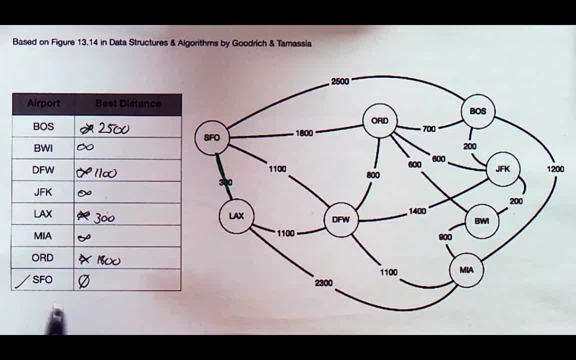 So it's got an edge back to San Francisco, but San Francisco is already connected, So there's no need to worry about that one. It's got an edge going to Dallas, So we'll go ahead and update that. So it's no better than this. 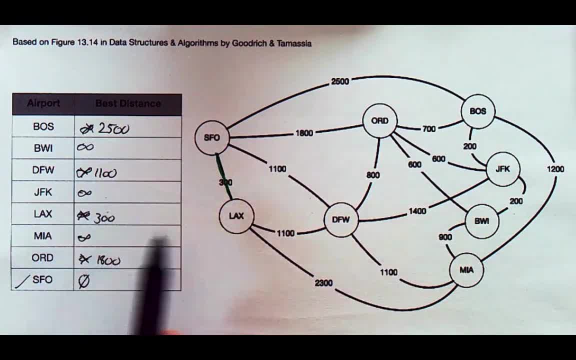 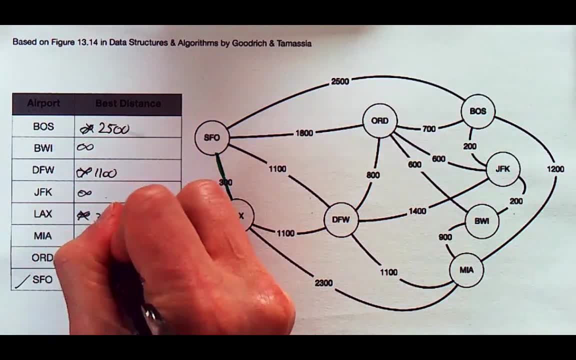 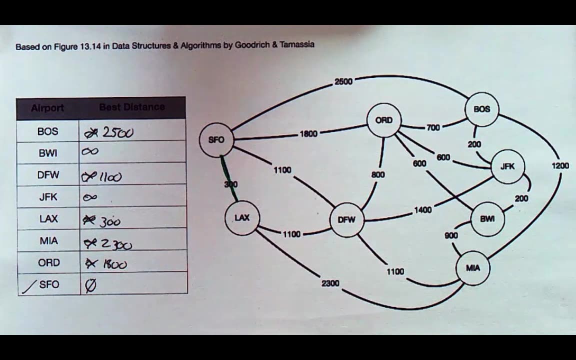 So we've got these two different options to get to Dallas with eleven hundred, And then there's an outgoing edge to Miami, So it's a total of twenty three hundred, which is better than infinity. So go ahead and add that in there. OK, so we've now processed LA. 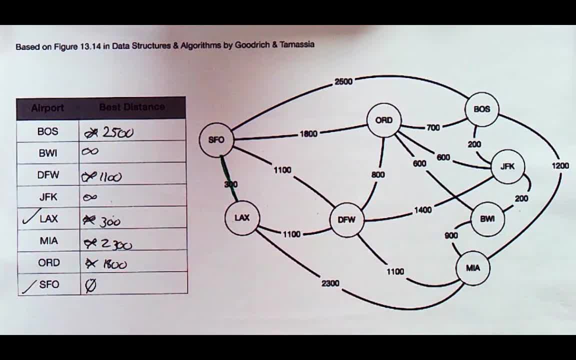 Now we're going to look at our minimum remaining item. So let's see twenty five hundred eleven hundred of infinity, infinity, twenty three hundred eighteen hundred. It looks like our trip to Dallas is our best choice. So, if you remember, we actually had two options to to get there. 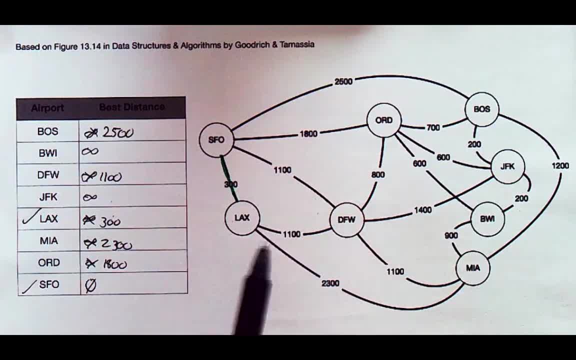 But this is the one that got added first And this one didn't didn't get added because it wasn't actually better. So I'm going to go ahead and indicate: Take that path to Dallas. Now we'll go ahead and process Dallas. So we'll look at all of the outgoing edges. 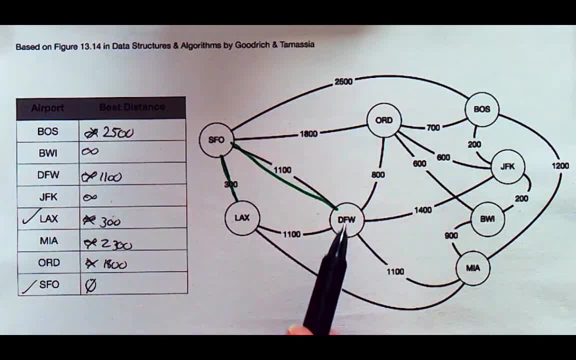 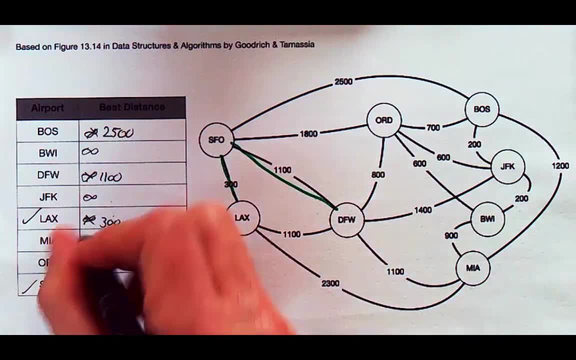 And again, I'm going to ignore if the opposite vertex is actually already connected. So we can get to Chicago O'Hare with a total of eight hundred. So we can get to Chicago O'Hare with a total of eight hundred. That's better than eighteen hundred. So I'll go ahead and update that. 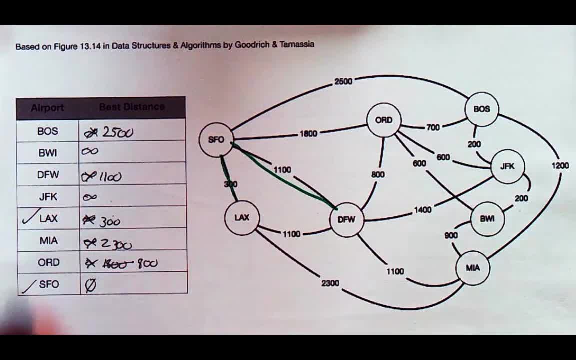 We can get to JFK with fourteen hundred. That's better than infinity. We'll update that, Let's see. we can get to Miami with eleven hundred. That's better than twenty three hundred. Update that, And we can get back to LA with eleven hundred. 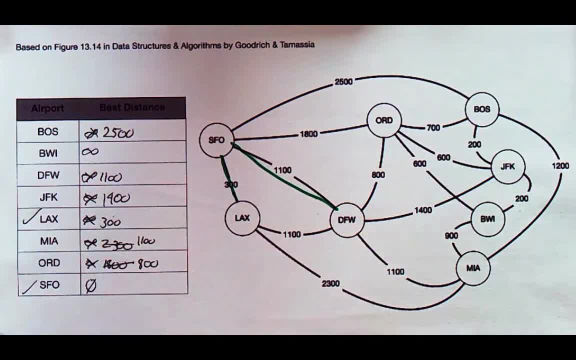 But LA was already connected, So again I'm going to ignore that. OK, so we're done with Dallas. So next we go through our priority queue yet again. So we've got eight hundred eleven hundred fourteen hundred, eleven hundred fourteen hundred, infinity and twenty five hundred. 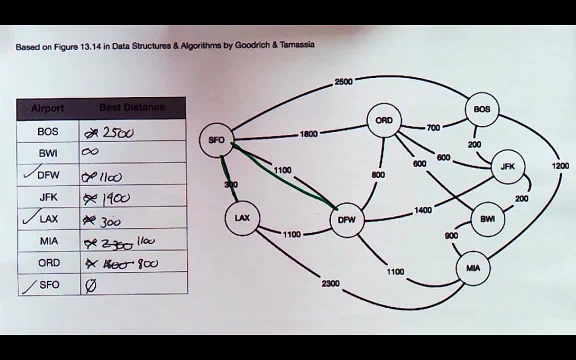 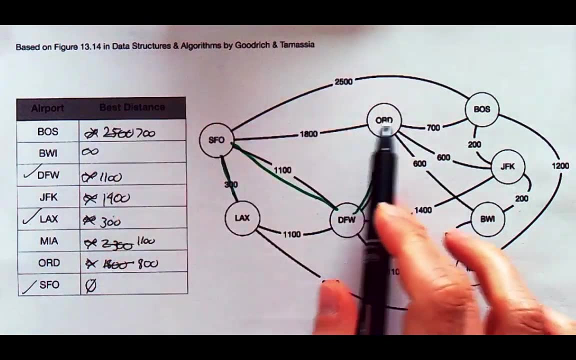 It looks like O'Hare is our best choice. So we'll go ahead and look at that. So we'll update our outgoing distances. So we've got an outgoing edge to Boston at seven hundred. That's a lot better than twenty five hundred. We'll update that. 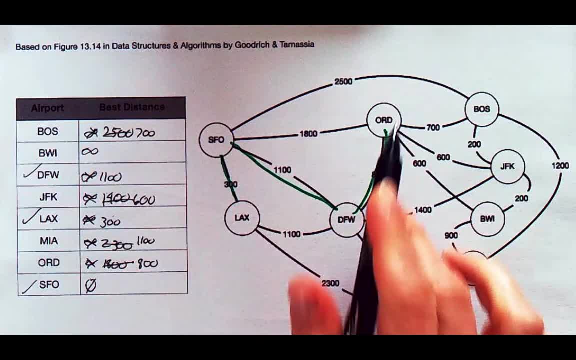 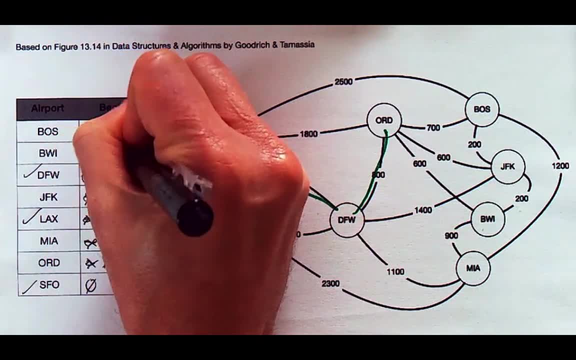 JFK at six hundred, So we'll update that. Baltimore at six hundred. Oh, it's better than infinity. Then we'll update that. That's great. We could go back to Dallas-Fort Worth, But again it's already connected. We could go back to San Francisco, but it's already connected. 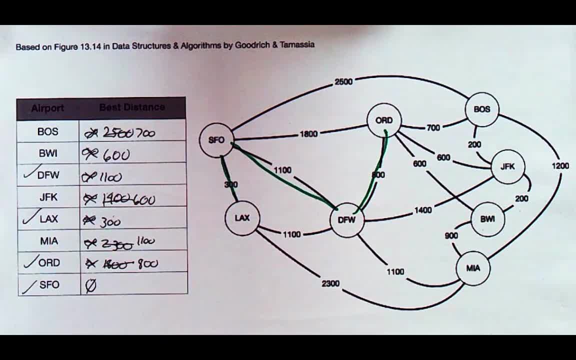 So at that point I'm done processing O'Hare. Looking down at our remaining vertices, we've got eleven hundred, six hundred, six hundred and seven hundred. So again we've got a tie here to O'Hare. We're six hundred apart. It's kind of arbitrary which of these we pick. 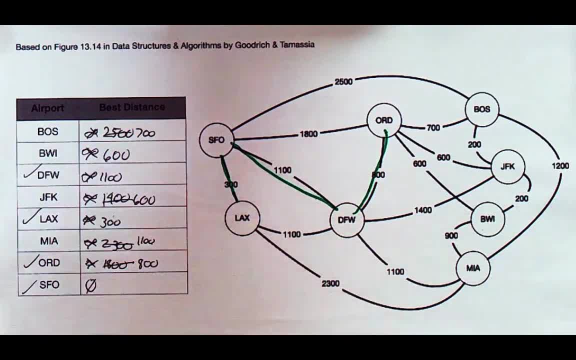 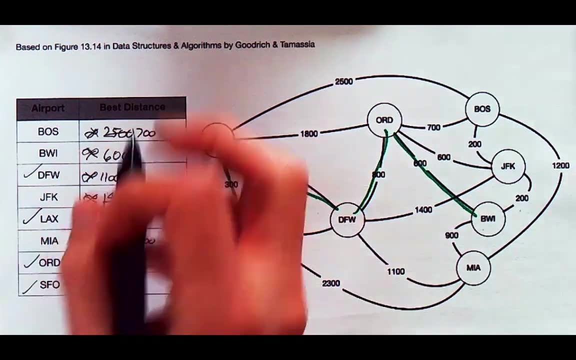 I'll go ahead and select Baltimore as our choice. So we'll highlight which edge got us there And then we'll go ahead and process Baltimore. So we've got an edge of weight two hundred going to JFK. That's better than six hundred, So we'll update that. 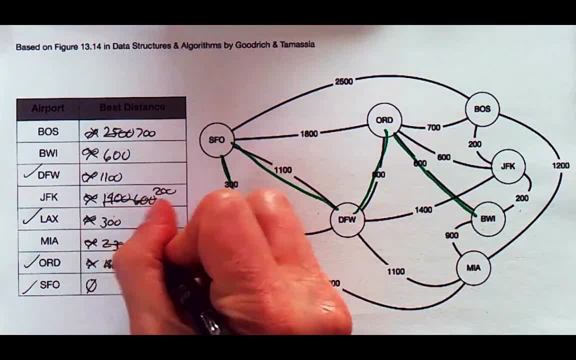 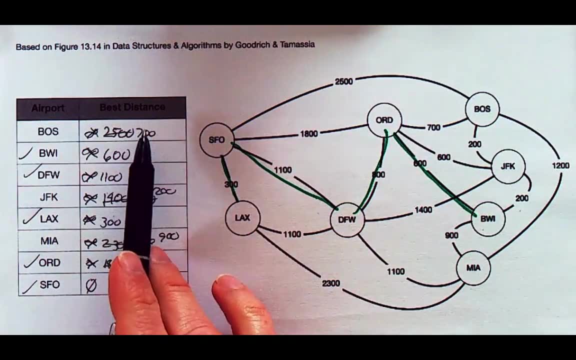 Then we've got an edge of nine hundred going to Miami. That's also better than our current estimate, So we'll update that And with that we're done with Baltimore. Looking through our priorities, we've got seven hundred two hundred and nine hundred. 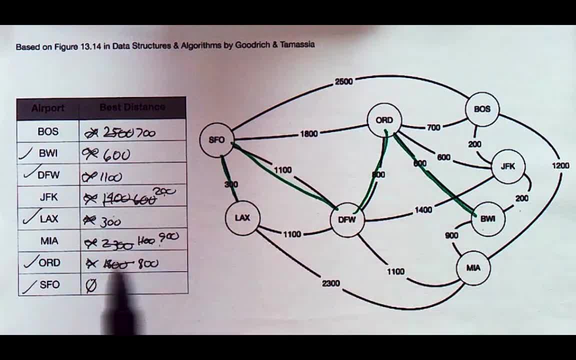 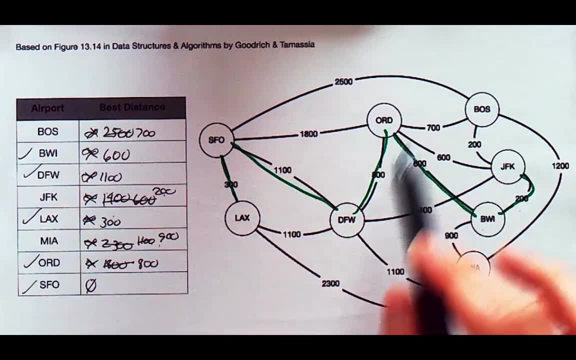 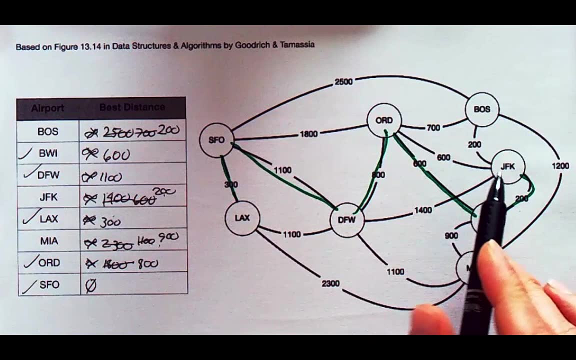 It looks like JFK is our best bet here, So we'll go there next. OK, so processing its outgoing edges. Two hundred to Boston, Oh, that's better than seven hundred, So we'll go ahead and update that Six hundred back to O'Hare. but that's already been processed.